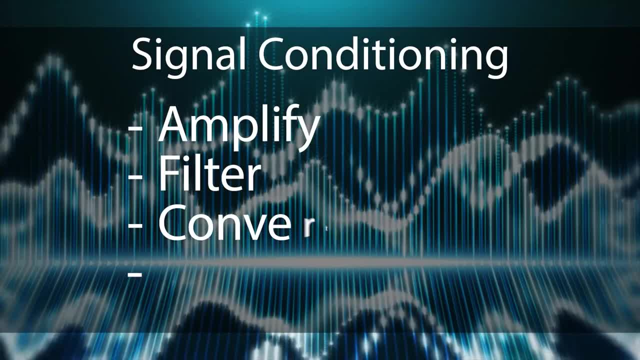 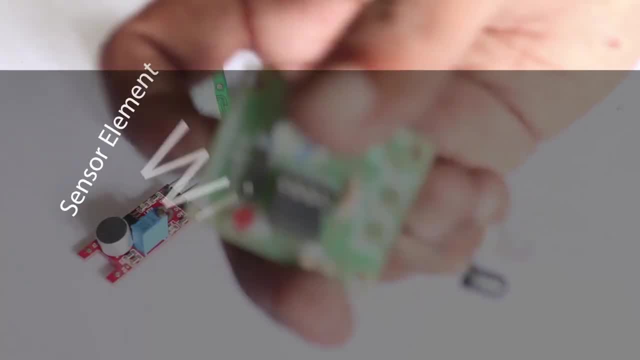 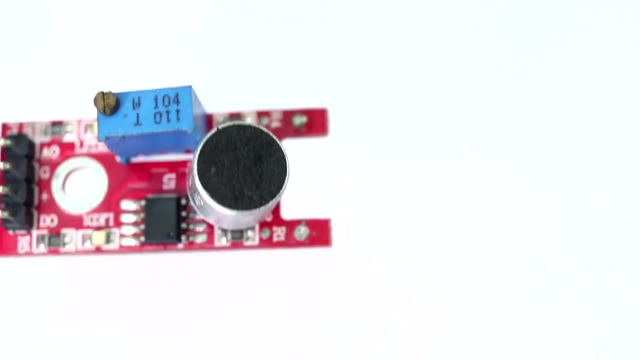 In such cases, a signal conditioning circuit is required in order to amplify and filter the signal produced by the sensor element in the desired range. with respect to the microcontroller, The sensor element and the conditioning circuit is together known as the sensor module. For example, in the case of a microphone, it detects audio signal and converts to output. 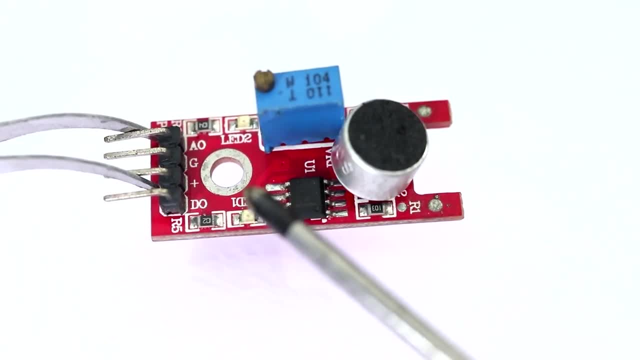 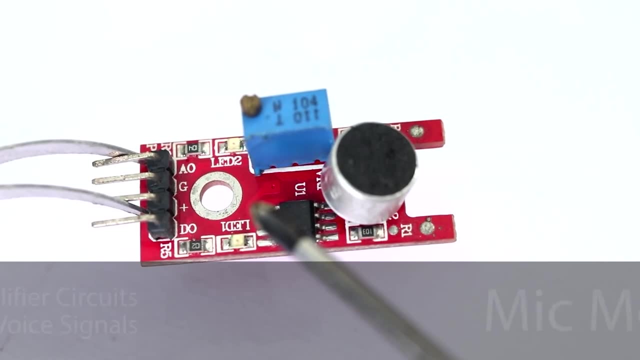 voltage, which will be in terms of V. This voltage is not enough to drive a circuit, So an amplifier will be used to increase the signal strength before using it in circuits like flap switches or feeding it to Arduino. Now you know how a sensor works. 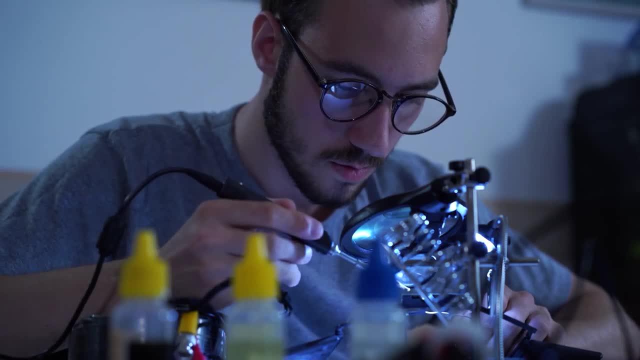 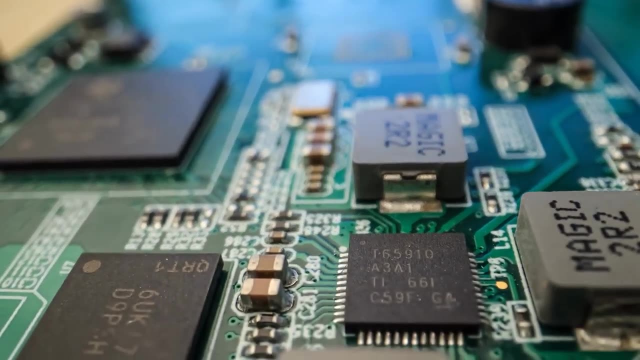 Let me tell you something interesting. You can create your own sensors with a few cheap raw materials. All you need is a sensor element and some cheap components to set up a conditioning circuit. You can even design and make your own sensor module boards using PCB designers like Altium. 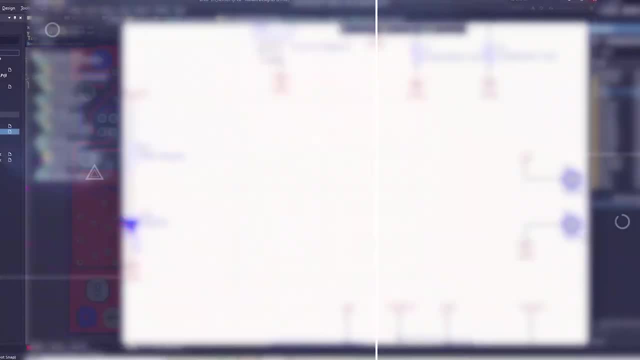 Altium is a PCB designer that can do this. Altium is a PCB designer that can do this. Altium is a PCB designer that can be used to create simple PCBs for your hobby projects or complex and multi-layer PCBs for industrial use. 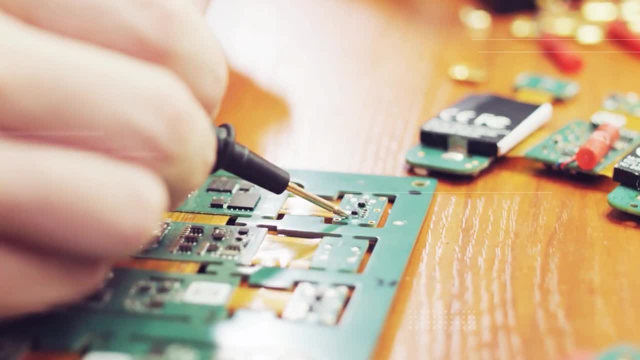 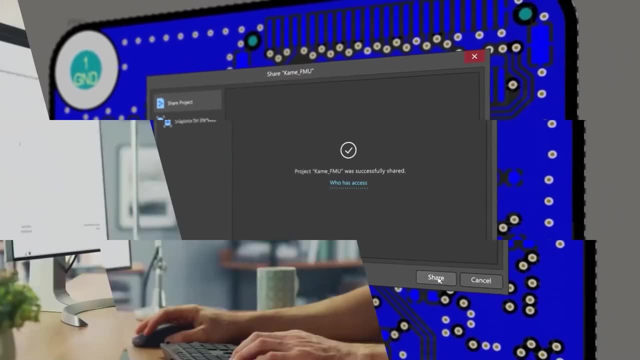 It's easy to create our own PCBs using Altium. If you are a DIY electronics enthusiast, you're gonna love it. Altium subscription includes something called Altium 365, which lets you design, share and manufacture your project in one place. 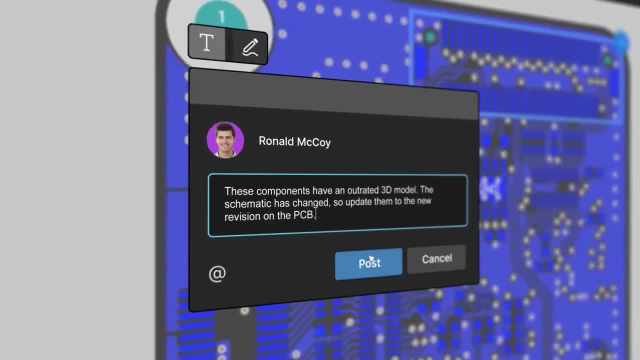 Secure, centralized cloud storage lets you share your designs and ideas with teammates or clients. You can download and install the free trial version from the description down below. Altium is one of the best sensors in the market. It's easy to use and it's easy to use. 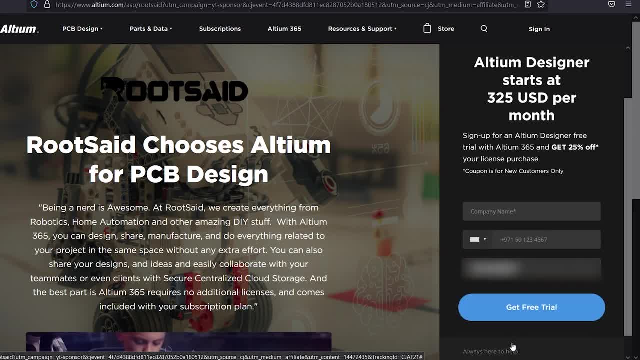 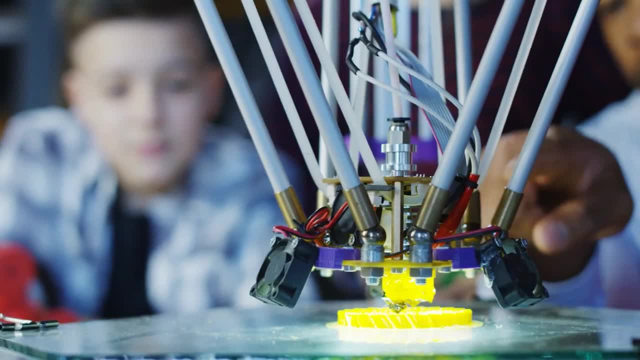 It's easy to use and it's easy to use. It's easy to use and it's easy to use, And if you are a student, you get a 6-month full license absolutely free. Don't miss out. This is basically how a sensor works. 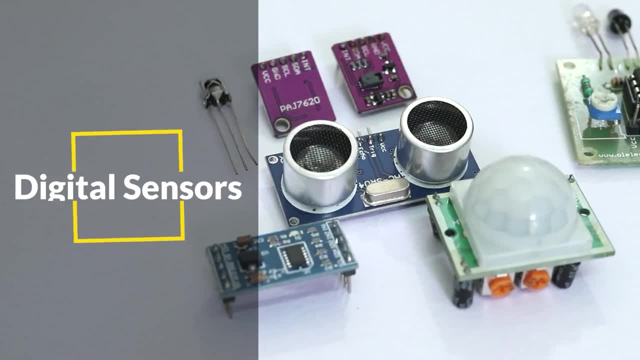 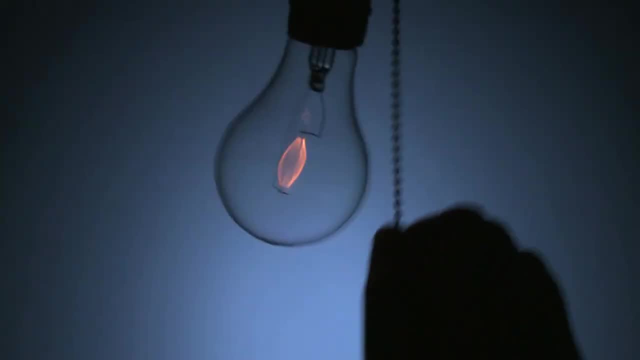 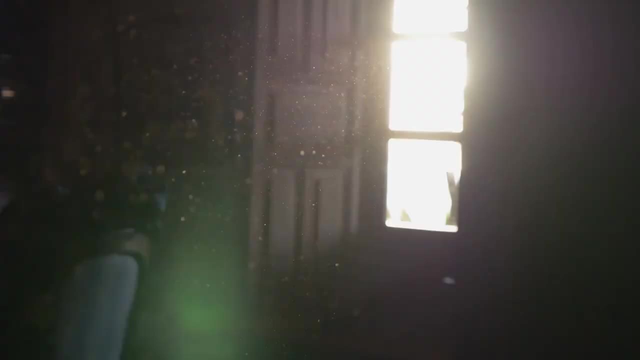 Based on the type of output signal. there are mainly two types of sensors: digital and analog sensors. Digital sensors are kind of like on-off switches: Either there is light or not, one or zero, true or false. But the world is not just zeros and ones, is it? 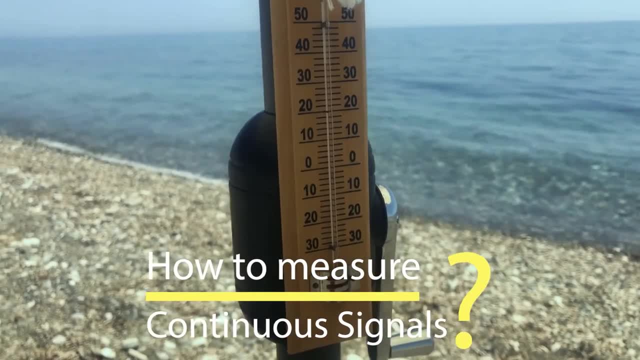 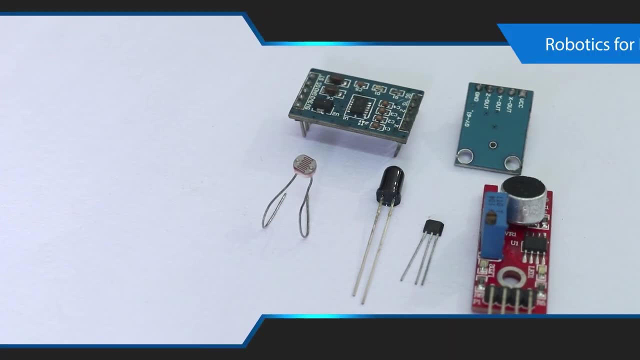 What if you want to measure ambient light using LED lights, Or temperature using a temperature sensor? What if you want to measure values between zeros and ones? That's where we use analog sensors. Analog sensors are very simple. It has a voltage output that can vary with respect to the external physical quantity. 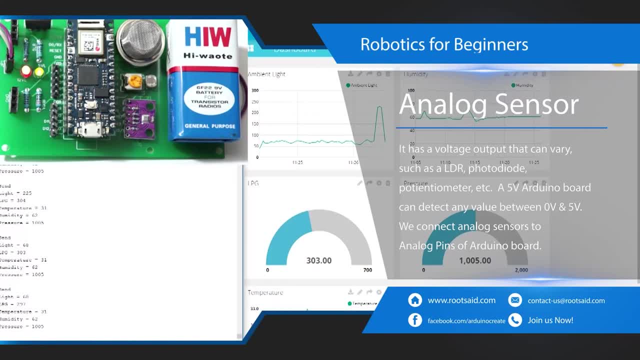 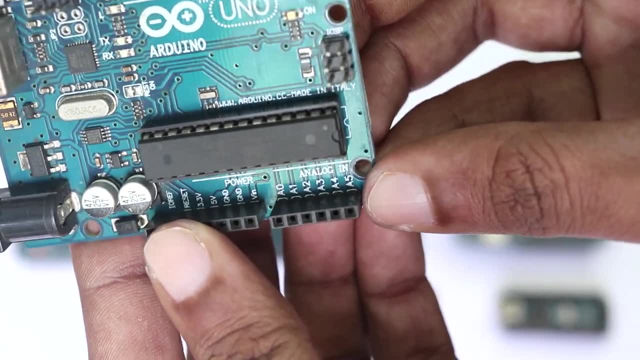 This way, you can measure the correct value of light, and not just black or white. Typically, the analog voltages are input to a microcontroller like Arduino via the analog pins. That being said, let me show you something that's really useful. 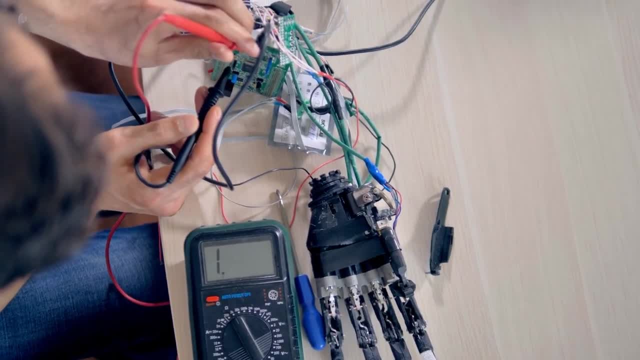 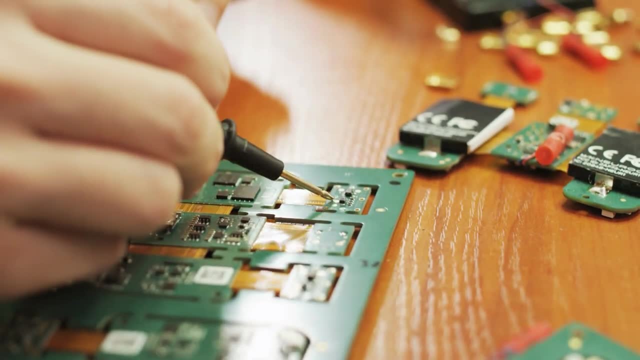 Before you start your project, buy your sensors or buy the components for making your own sensor, It's always a good idea to have a good knowledge of the sensors and components, such as specifications, availability, as well as the price. For that, I would recommend this free site called Octopart. 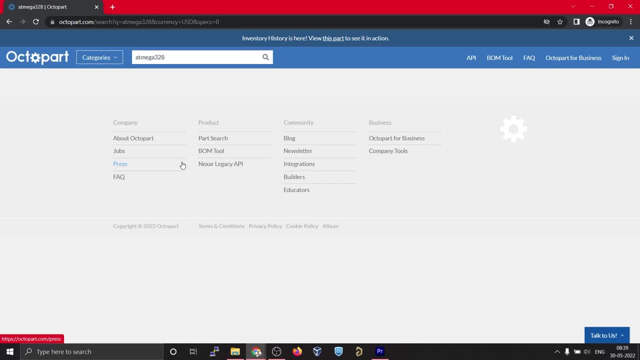 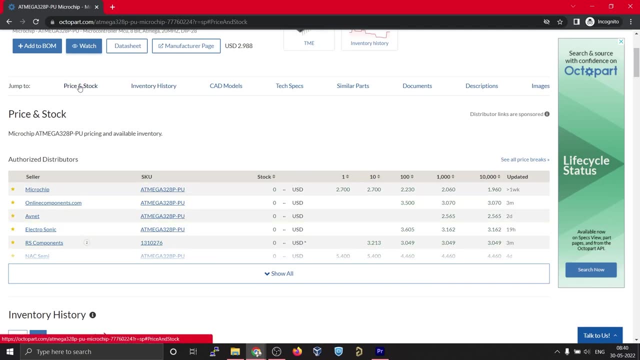 Octopart is an amazing electronic component search engine. You can use Octopart to figure out from where you can buy your components, the price as well as the availability. You can also use Octopart to find sensors that meet your requirements. 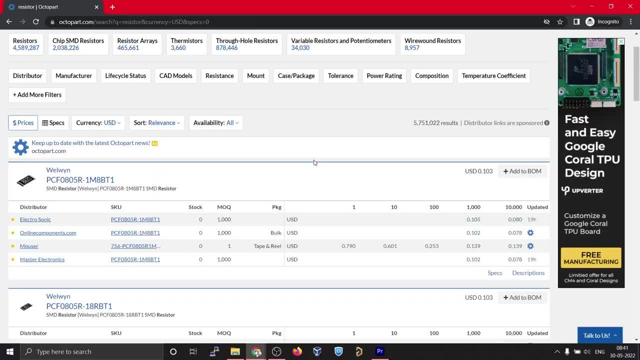 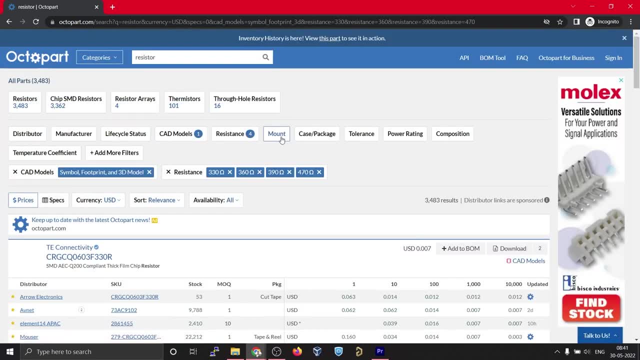 You can even purchase the components by simply clicking the link here itself. It's a free solution for most of our problems and you will get everything in one place. This is also going to be really useful for you guys, so make sure you check it out. 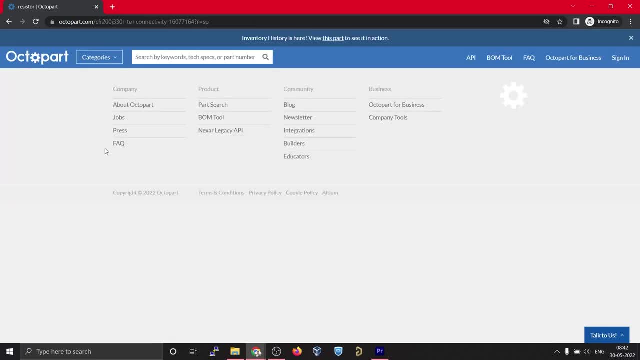 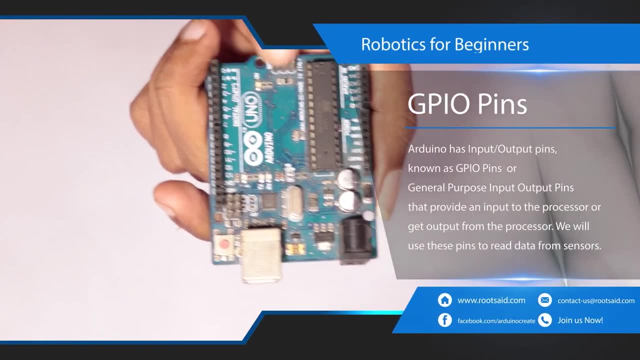 We now have measured the physical quantity and convert to its electrical equivalent. All we need to do is read it with the help of an Arduino and do something useful. Arduino has several input output pins, generally known as GPIO pins or general purpose input output pins. 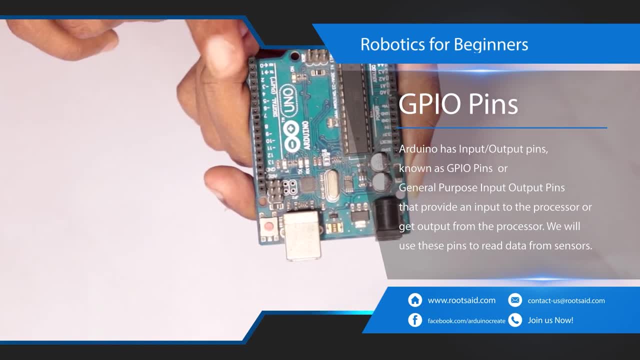 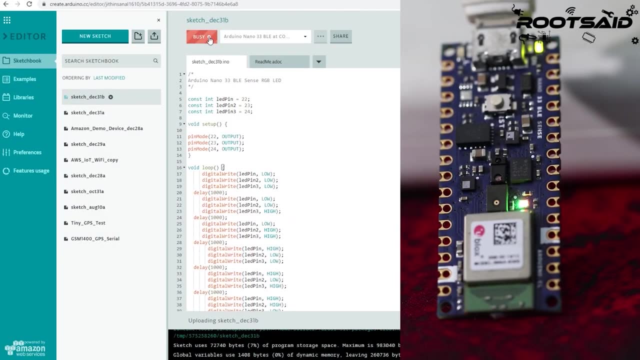 These pins are designed either to provide an input to the processor or get output from the processor. We will be making use of these pins to read the data from the sensors. Microcontrollers in Arduino boards are capable of detecting binary signals or digital signals 0 or 1.. 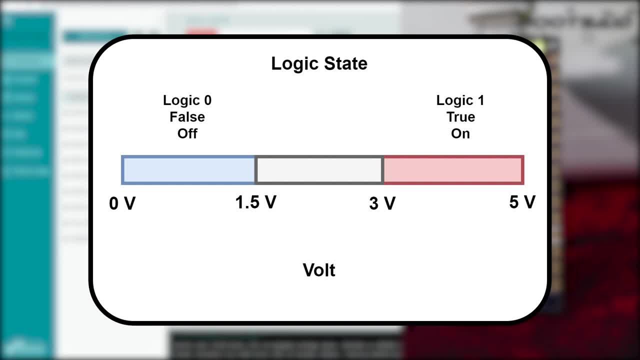 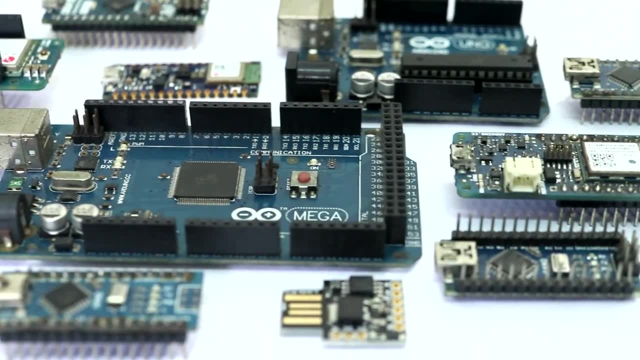 That is for a 5V Arduino board. it understands 0V as logic 0 and a voltage above 3V as logic 1.. In most of the boards almost all the GPIO pins in Arduino can be used as digital pins. 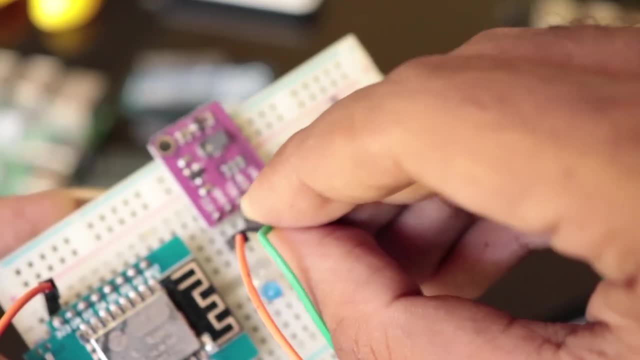 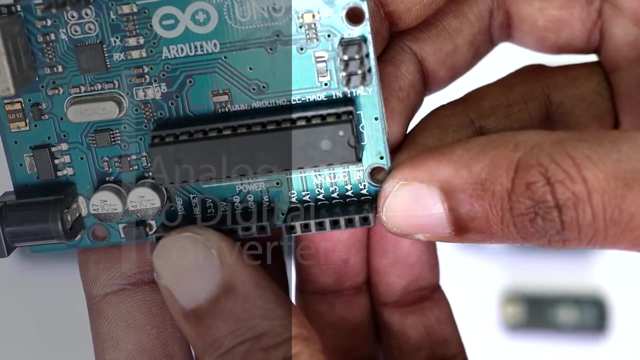 which means it can be used to connect digital components To measure the value of analog signals. the Arduino has built-in analog-to-digital converters at certain pins. These ADC circuits turn the analog voltage into a digital value which the Arduino can read. 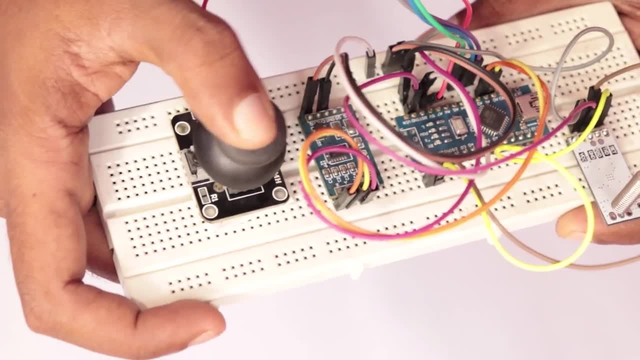 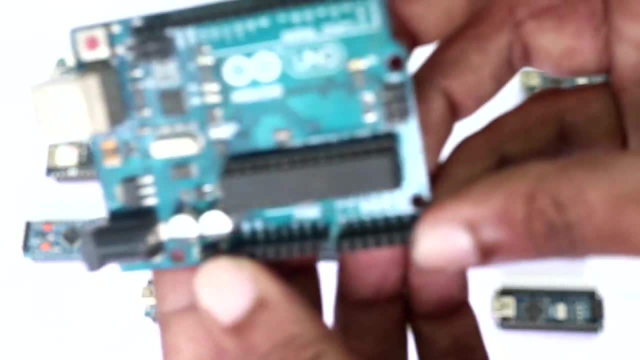 These pins are what we call analog pins. This is where we connect the analog sensor input. Different boards will be having different number of analog pins. For example, Arduino Uno has 6 analog pins, A0 to A5.. Let me know how many analog pins you know. 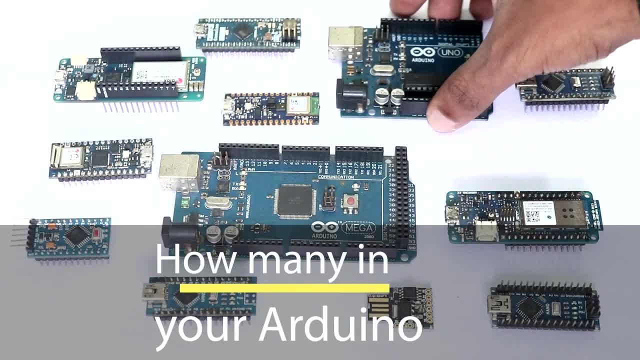 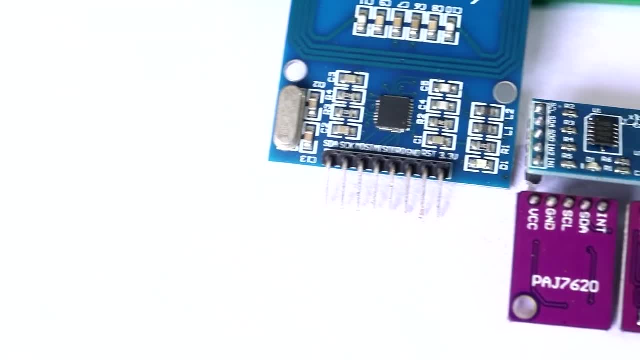 I will try to figure out how many analog pins you know. Let me know how many analog pins you know. Let me know how many analog pins you have in your Arduino board. Simply comment the board name and the number of pins. Within the category of digital sensors, there is another set of sensor modules whose output 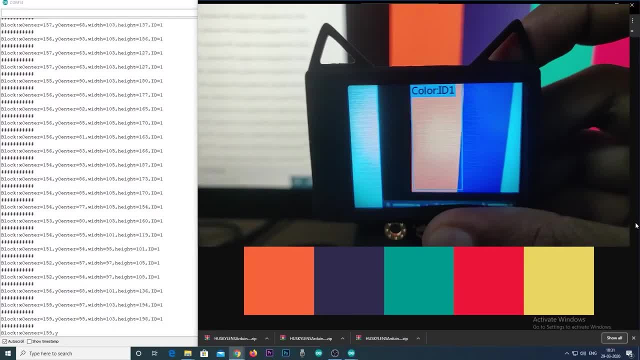 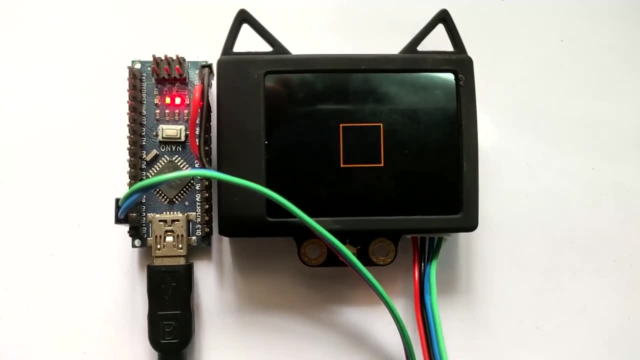 is available in the form of data transmitted via certain serial protocols like UART or I2C or SPI. Such sensors are interfaced to the communication channels to receive data using the microcontroller. Using these sensor outputs, we can write conditions in your Arduino code and upload it to your 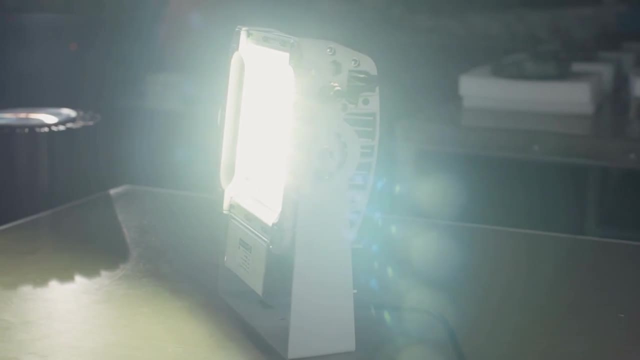 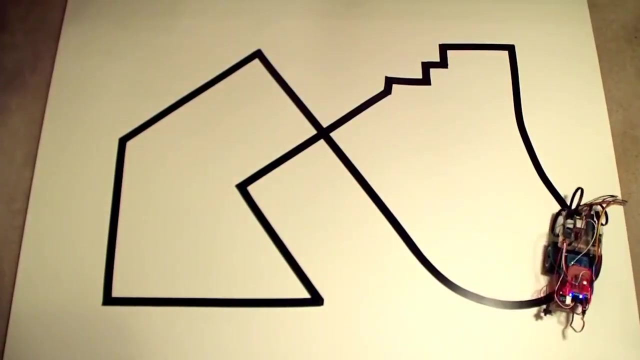 Arduino board. There are two fun stuff like turning on a bulb when ambient light is low or making an autonomous robot like a line follower which will sense its path using IR sensor and follows the line. I have a list of sensors which are beginner friendly, easy to get started with and very 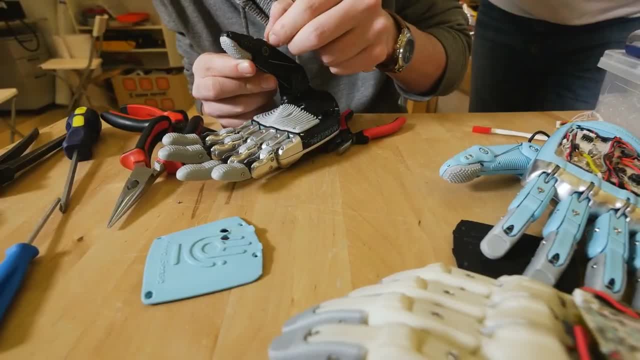 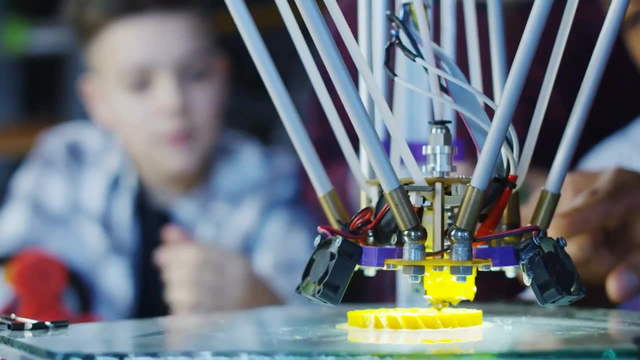 easy to hook up with Arduino and learn. it's working. So, if you want, I will leave the link in the description. Let me know in the comments if I missed any beginner friendly sensors. Now, as usual, an example. Consider this line following: robot using Arduino. 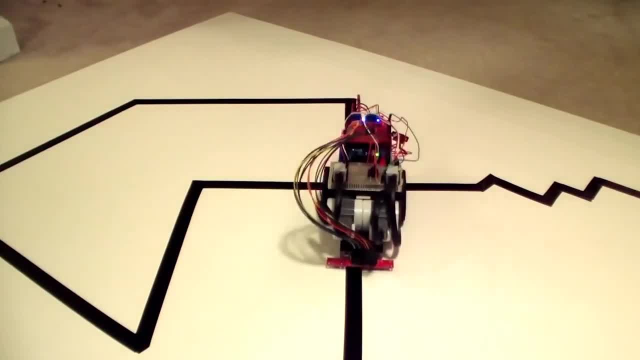 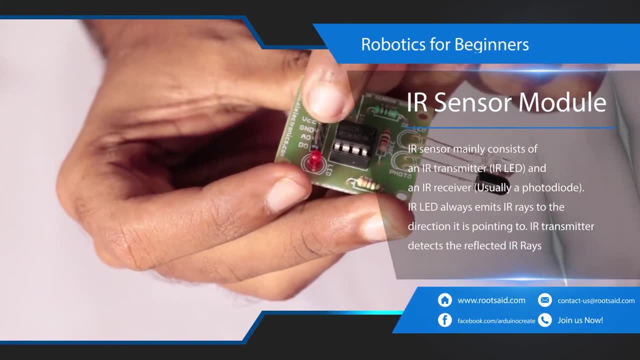 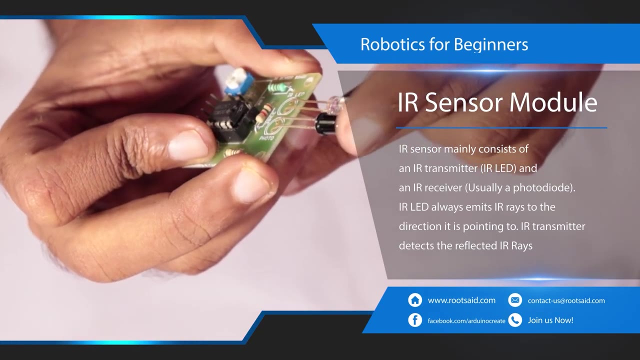 This robot uses IR sensor to detect the track and use motors to move around depending upon the color of the track. Here, IR sensor is the sensor that senses the environment and gathers input. IR sensors mainly consist of an IR transmitter, an IR LED and an IR receiver, usually a photodiode. 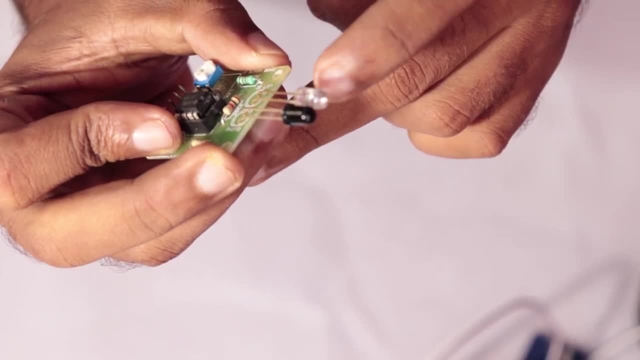 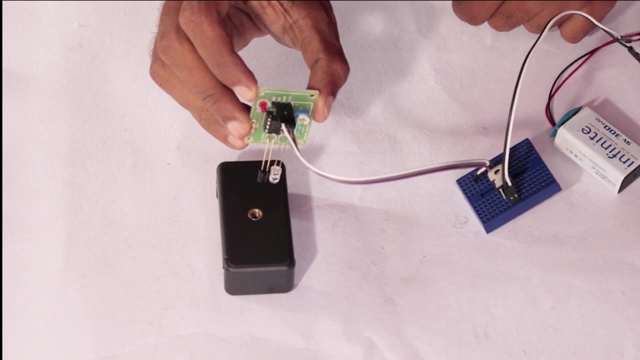 IR LED always emits IR rays to the direction it is pointing to. Now let us bring it closer to a surface. When the IR rays hit a surface, some rays will be reflected back depending upon the color of the surface, Which means the brighter the color is, the more IR will be reflected back.